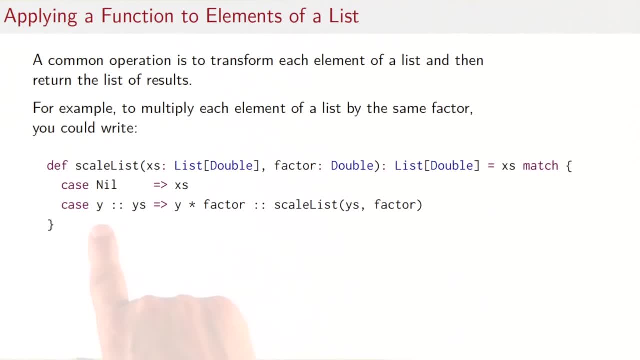 is nil, it just returns it unchanged And otherwise it multiplies the first element of the list by the factor and it does a recursive call of scaleList with the rest of the list and factor. So obviously that function would multiply each element of the list by the same factor. 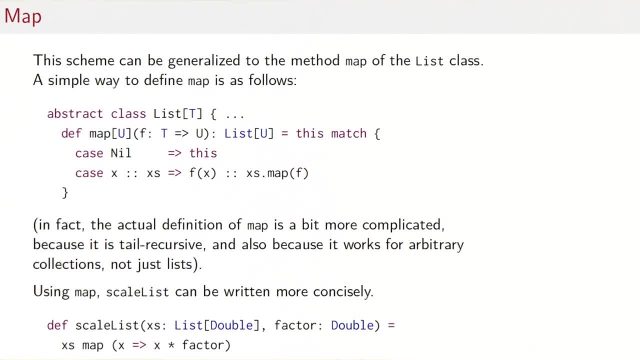 That scheme can be generalized to a method, map on the list class, which can apply an arbitrary operation to all elements of a list. So here's a simple way to define map on the abstract class list of t. We would say def map and map takes a. 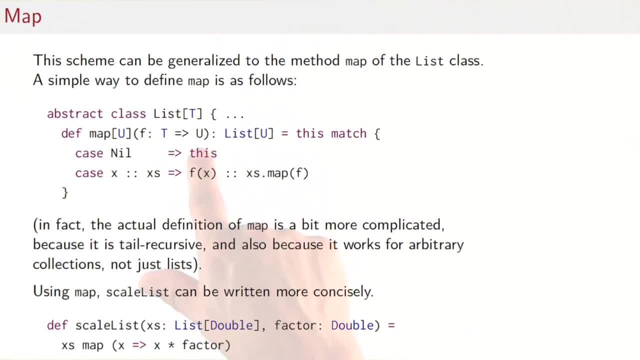 function from t to some other type u, which could be the same as type t or it could be different. So u is a type parameter of map and then it returns a list of u And then the body of map is just like the. 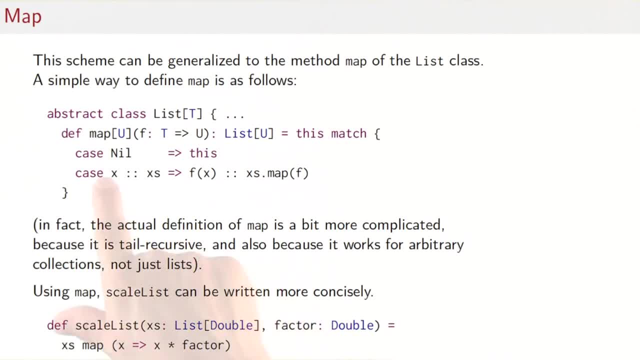 body of scaleList, but now generalized. So in the case of nil we return the list unchanged. If the list is non-nil, then we apply the function f to the first element, x, and we follow that with a recursive call of xsmap. 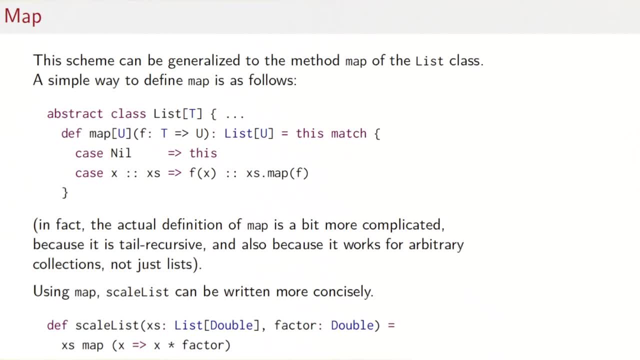 In fact, the actual implementation of map in class list in the Scala standard library is a bit more complicated, for several reasons. First, the actual definition is in fact tail recursive, whereas this definition isn't. You see, after the call to map we still have a call to cons. And second, the actual 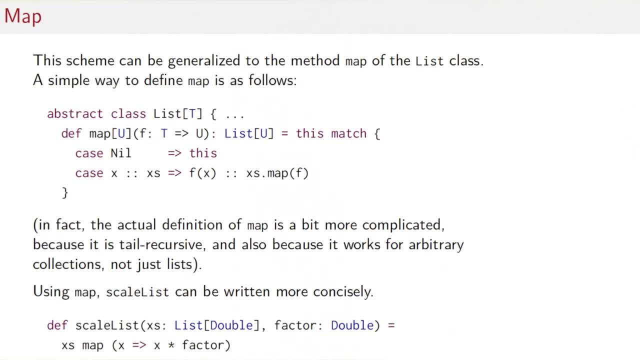 implementation of map works for arbitrary collections, not just lists, But for understanding map, this definition here will do very well. So using map, we can now write scaleList much more concisely- so much more concisely that it's hardly worth writing a different function for it. 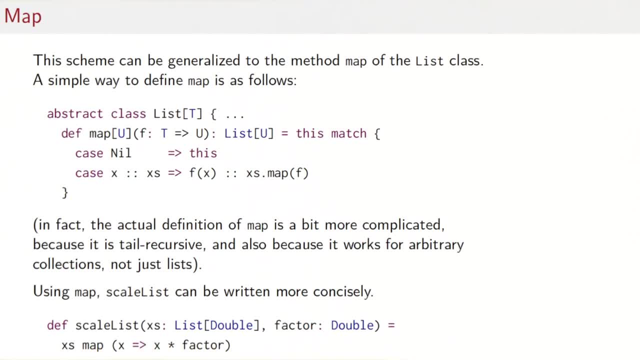 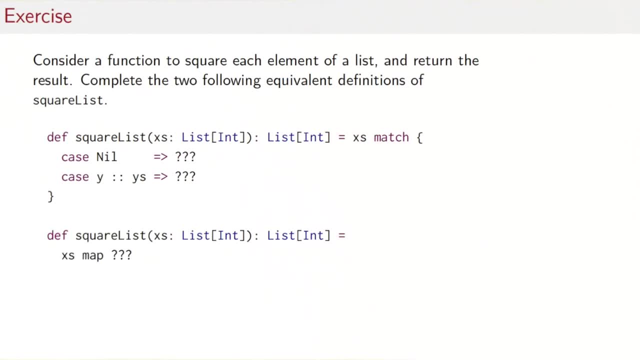 We would just say scaleList of xs, and the factor is map, xsmap, with the function that takes an x and multiplies x by the factor. So here's an exercise for you. Let's take a function, squareList, that squares each element of a list and 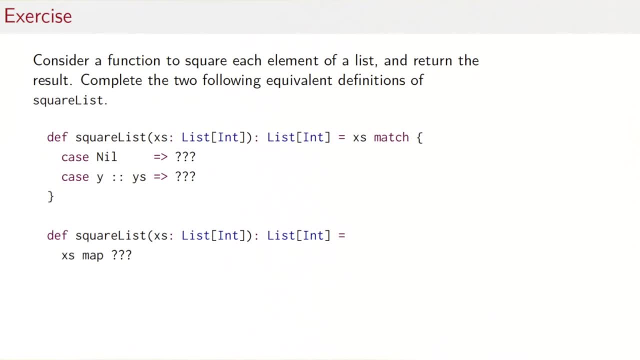 returns the result. There are two possible ways to do that: either with pattern matching or using map. I invite you to try both possible ways by filling in the three triple question marks in the definition of squareList here and the definition of squareList down there. So let's see how we would do that In the 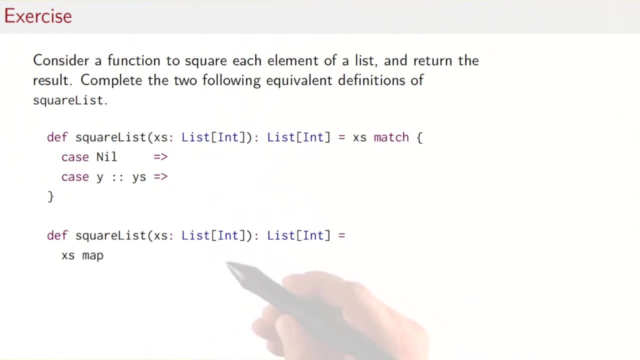 pattern matching definition. to take the squares of an empty list, we would surely return the empty list again. To take the squares of a list with a head y and a tail ys. what do we do? Well, we start by taking the square of y and we follow that. 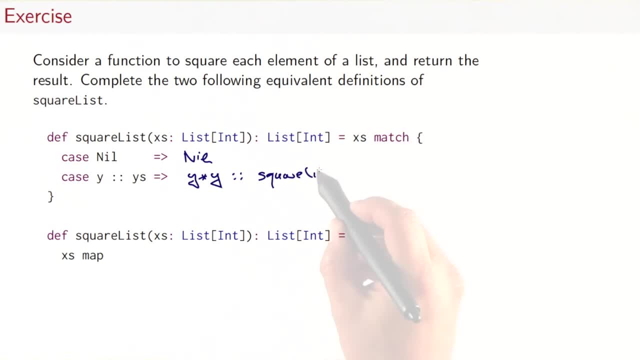 by a recursive call of squareList of ys. So far, so good. I think by now we all know how to do these things cold. But let's see whether we can do that, So we can do it shorter using map. Well, to use squareList with map, what can we do? 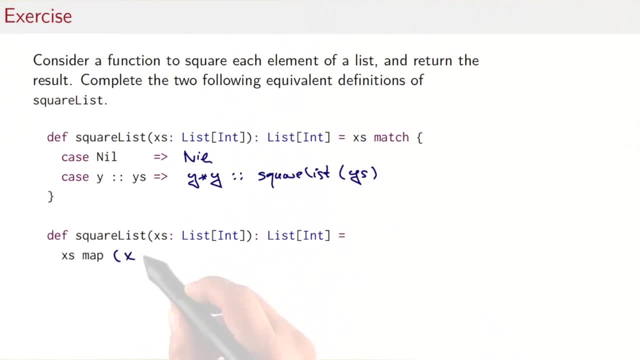 Well, we map it by the function that takes an x and returns x times x, And that's it. So obviously the definition with map is much shorter and, I would argue, also clearer than the one that uses pattern matching and recursion. So here's another common operation. 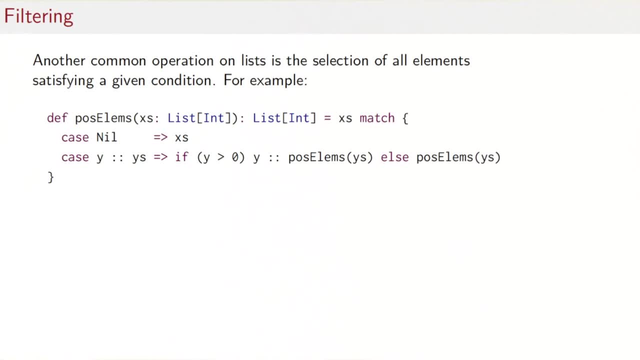 On lists selecting all elements that satisfy a given condition. For instance, you might want to select all elements from a list that are positive. Here you have a function: posElements. It takes a list of int, gives you back a list of int. 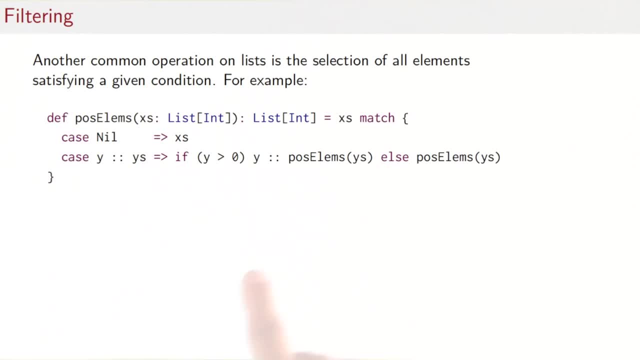 And the pattern matching definition would read as you see here. So for the empty list, we can just return it. If it's nonempty and the first element is in fact greater than zero, it's positive, then we include it in the result. 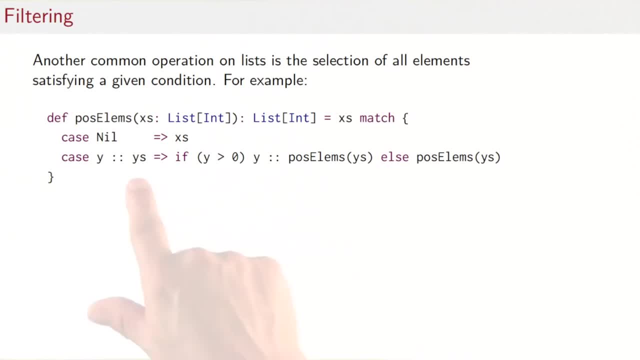 So we return the first element followed by posElements of the rest of the list, And otherwise we just do posElements of the rest of the list. So the first element gets dropped and we just filter the remainder of the list with posElements. 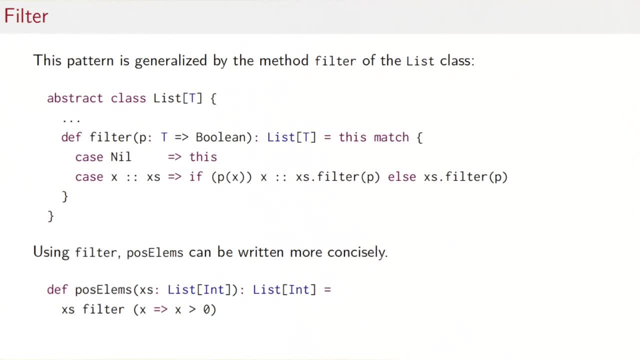 Again, this pattern can be generalized to a method filter in the list class. So here you see the definition of filter. It takes now a predicate that takes an element of the list element type And it gives you back a Boolean And it will return a list of t's. 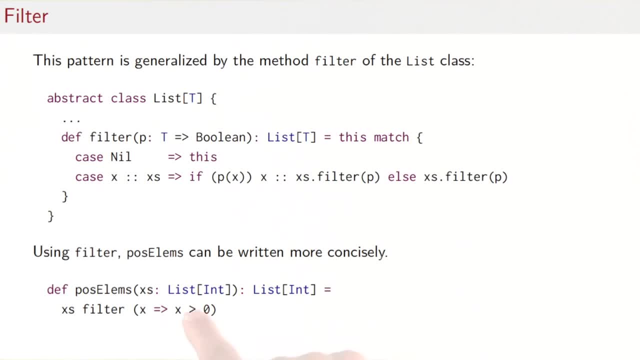 The definition is an obvious generalization of posElements that you've seen before. So we match on the current list. If it's nil, then we return the nil list. If it's not nil and the head of the list xs satisfies our predicate. 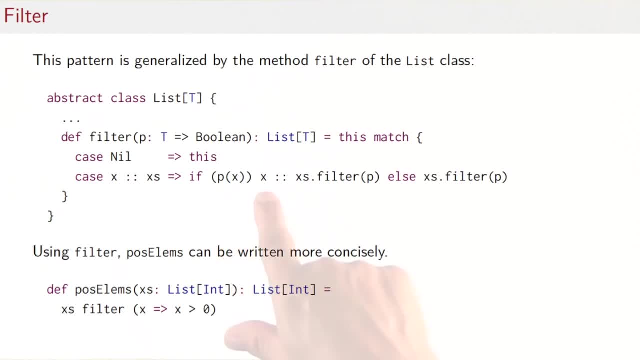 So p of x is true. Then we return x, followed by xs dot filter p And otherwise just xs. Again using filter, we can write posElements much more concisely. We would just write xs, filter x, such that x is greater than 0.. 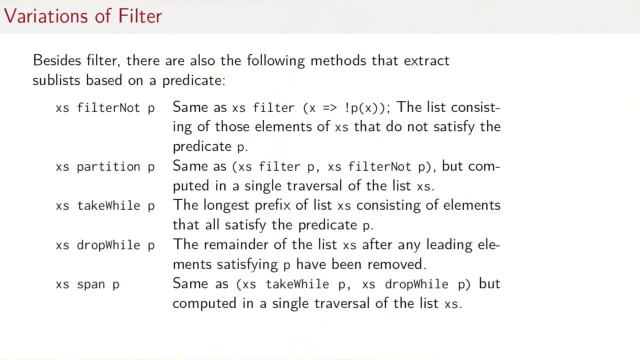 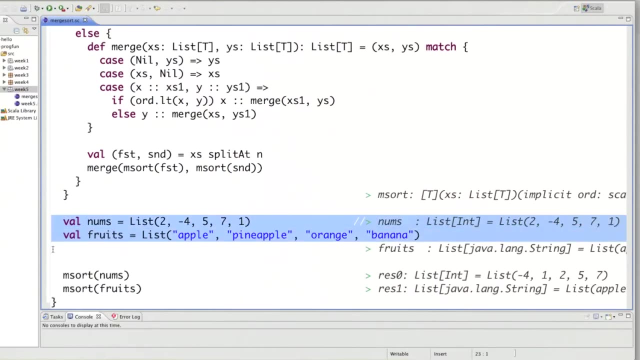 Besides filter, there are also other methods that extract sublists from a list based on some predicate. You see the list of these methods here. Rather than going through the list, I just wanted to show them in action in a new worksheet. So what I'm going to do is I'm going to take the data definitions of the previous worksheet. 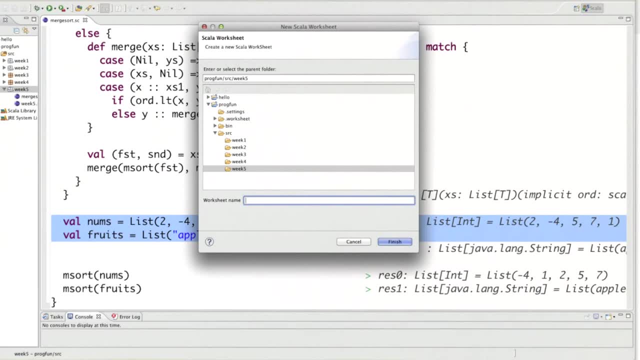 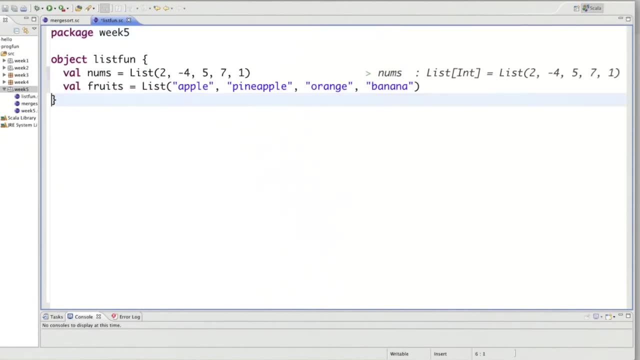 and create a new worksheet, call this list fun, And we have our test data here And what I'm, what we're going to do is, let's say, the first one would be nums filter. Okay, Okay, Okay. So all numbers greater than 0.. 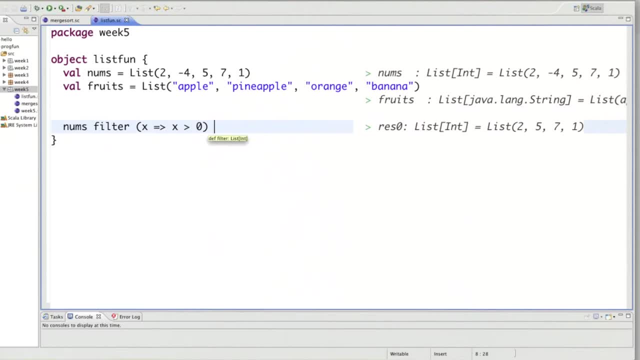 So that would have filtered out the minus 4 here. If we do nums filter, not x, x greater than 0, what do you expect to get Right? You'd expect to get just the negative number minus 4.. The other method was partition. 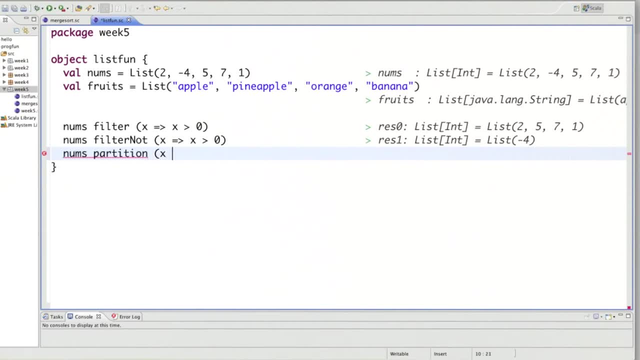 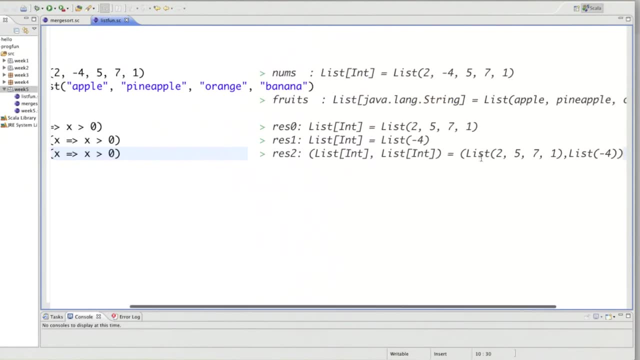 Partition is like filter and filter, not in one go. So If you write that here, Then what you see is you get a pair of two lists. The first list contains all those elements for which the predicate here is true. So that was the positive elements. 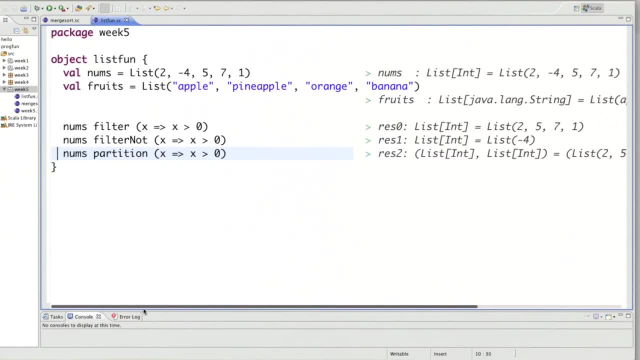 And the second list contains all those elements for which the predicate is false. So you see that partition is just like filter and filter, not as a pair. However, it will run in a single traversal through the input list numbers, Whereas if you do first a filter and then a filter not, you would get two traversals. 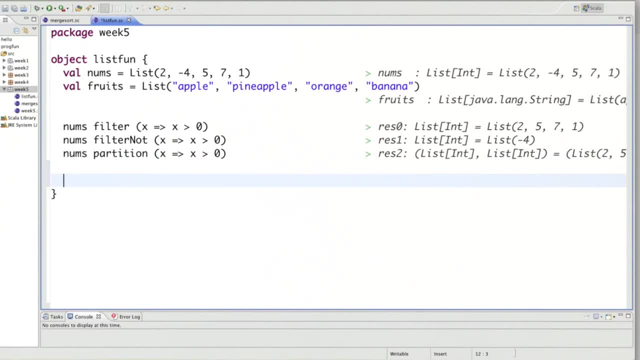 The next two functions are a bit different in that they look at a prefix and a suffix of a list. So what I can do here is I can say: nums take while x, x greater than 0. So what that gives me is the longest prefix of the list, such that the predicate is true. 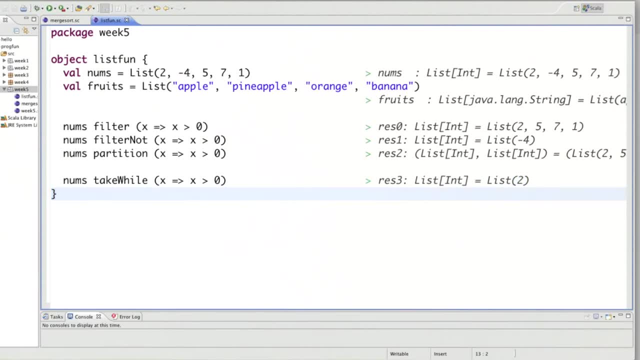 So here I would say: okay, 2 is greater than 0. But then at minus 4, I would stop because minus 4 is not greater than 0. So it will. any further elements will not take part in take while. 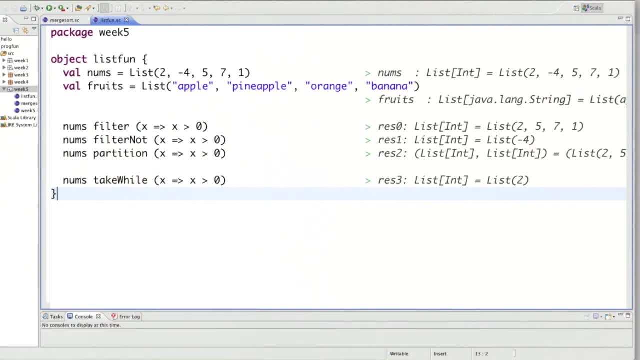 That's the main difference between take while and filter. Filter will always select all elements in the list that satisfy the criterion, Whereas take while will only take the longest prefix of the list. The opposite of take while is drop while, So So let's write that. 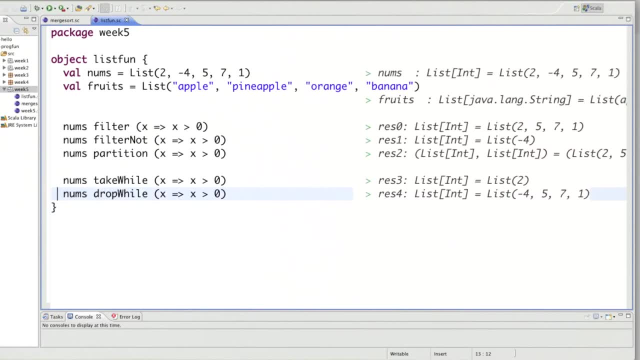 So take while and drop while relate to each other, just like take and drop relate to each other. Drop while would then return the remainder of the list without the prefix taken by take while. So it would be the list that starts with a negative element and then goes until the end. 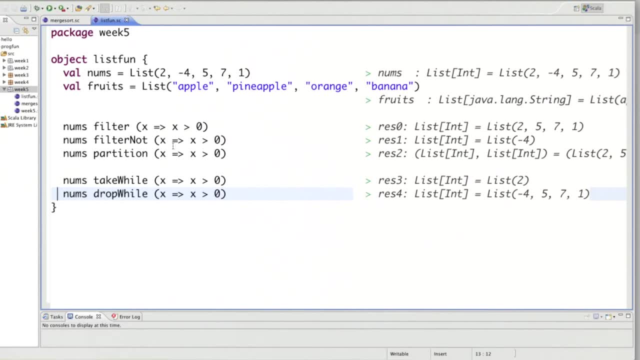 of the input list And, finally, where we had partition That combined the filter and filter not. We also have an operation that combines a take while and a drop while. That operation is called span. So if we do that, then what we will see is that it will give us essentially the combination. 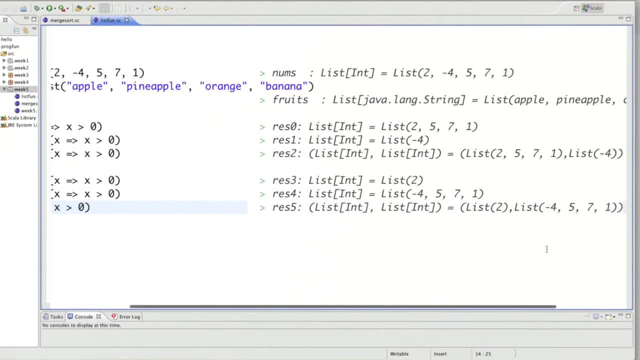 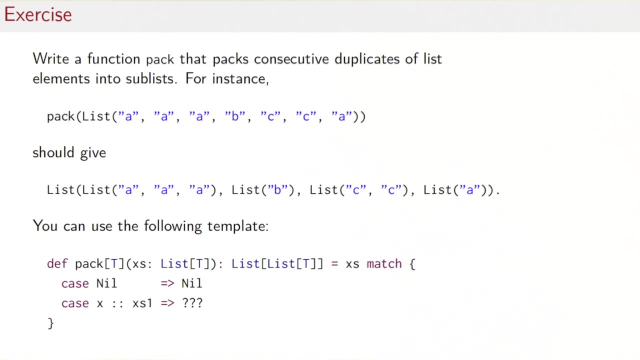 of a take while- that was the list 2- and a drop while, But like partition, it will only need a single traversal, not 2.. Let's apply the function that we've seen so far in an exercise. The task is to write a function pack. 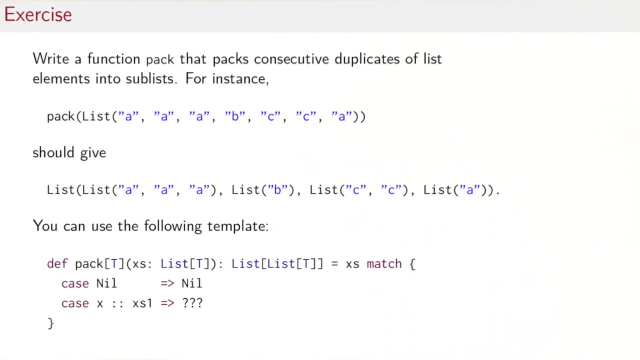 That packs consecutive duplicates of list elements into sublists. So if we apply pack to this input list here, we would expect to get back a list of lists where the first sublist is formed from from the three consecutive A's. here The second sublist has just a single B. The third sublist has the two consecutive C's. 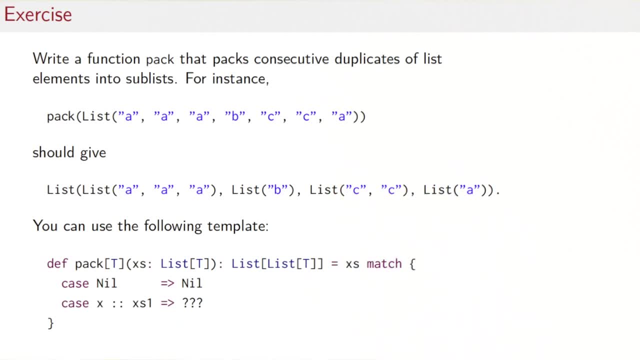 and the final sublist has the trailing A. here The idea is to use a template like this one here We have a defined pack to be. a generic function over type lists of T returns a list of list of T. Obviously, if the list is empty, then that's what we would expect back. 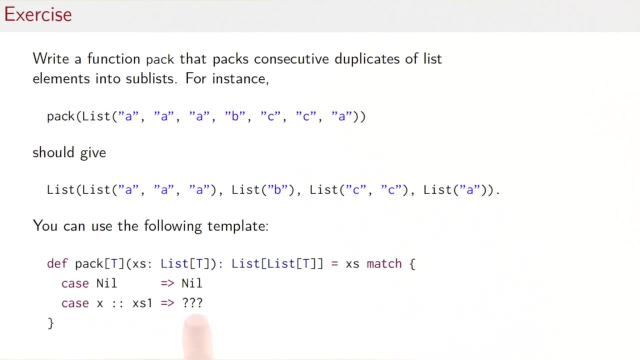 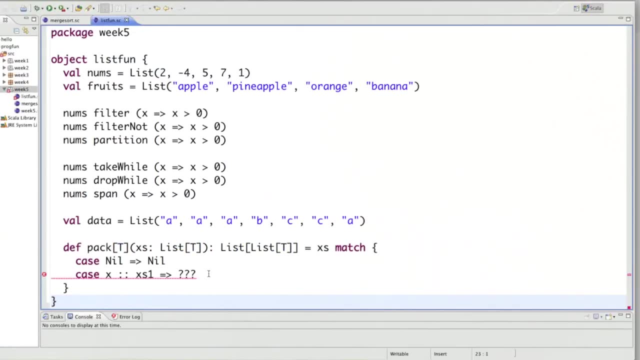 So the only case to handle is really this case here. If the list is nonempty, what do we do? I've already copied my input list data and the template of the pack function, though the only case to fill in is when the list is nonempty, consisting of a head, X and a tail. 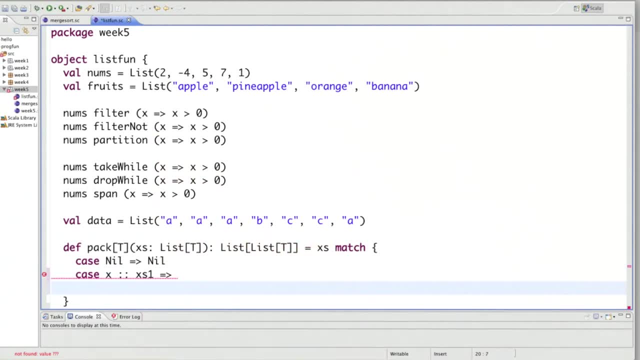 XS, Which of the six functions here would be applicable? Well, what we want to do is take off a leading sublist and then do something with the rest of the list, So it's a combination of take while and drop while, And that's what span would give us. 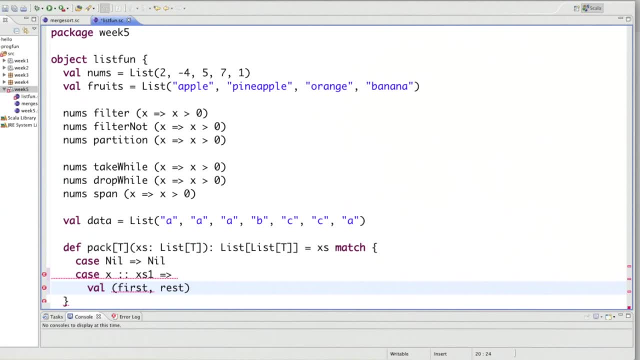 So let's set up a pattern: match first rest equals XS span. And what should the predicate be? Well, we say: take elements as long as they are equal. So let's say: take elements as long as they are equal to X, the leading element of the list. 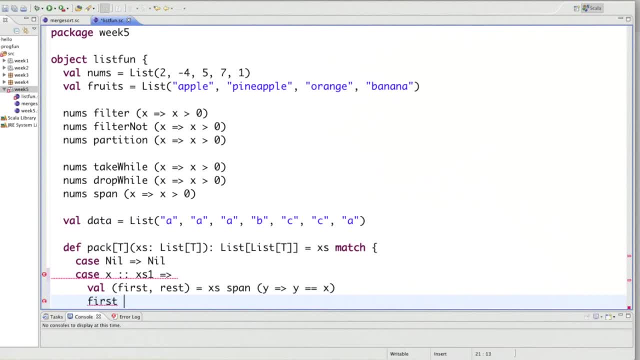 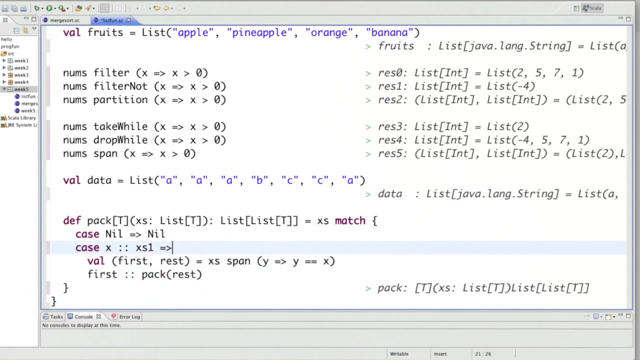 Once we have that, we would say first is already the sublist- that will constitute the first element of our list And the other elements would be the result of a recursive call of pack to the rest of the list And that gives us our function pack. 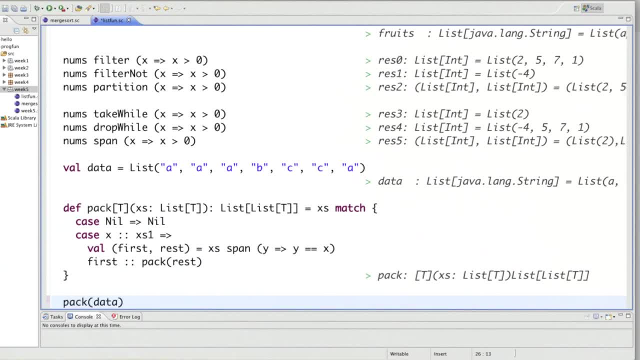 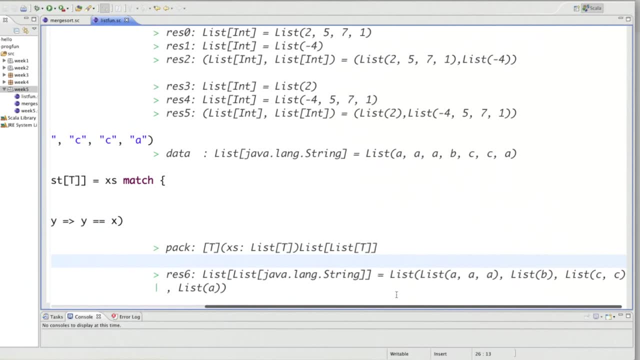 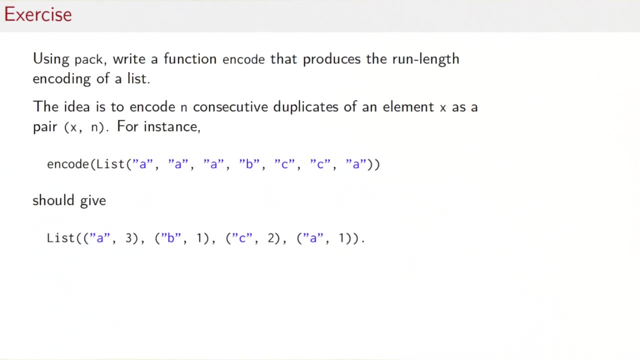 To our data list. pack of data gives us a list consisting of three A's, one B, two C's and an A- just what we needed. We're not done yet. As a second exercise, I would like you to use pack to write a second function- encode- that produces a run length encoding of a list. 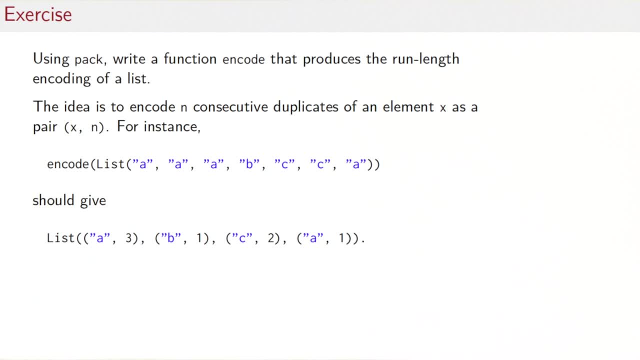 Run length encodings are often used for compressions of images and other files. The idea is to encode N consecutive duplicates of an element in the list as a pair- XN. So instead of writing the element N times, we just have a single entry, which is a pair of what the element was and how many times we have written it.